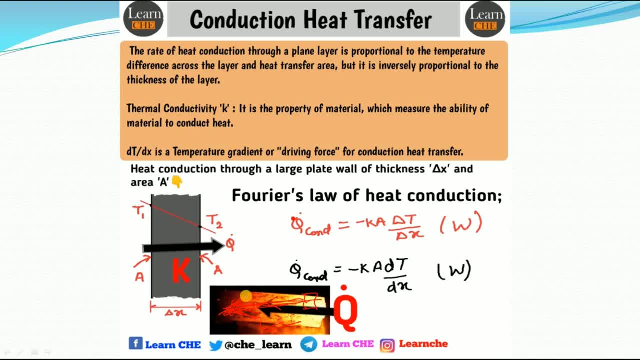 Okay, So this is an example of conduction, and you can also see the example of conduction in your home when you keep utensil on a stove or gas and you see that the handle of that, that utensil, becomes hot after some time. This happens because of the conduction where the more energetic particles transfer into the less energetic particles region, Right? So to define the conduction- heat transfer- we use a Fourier's law of conduction. What Fourier's law of conduction is? 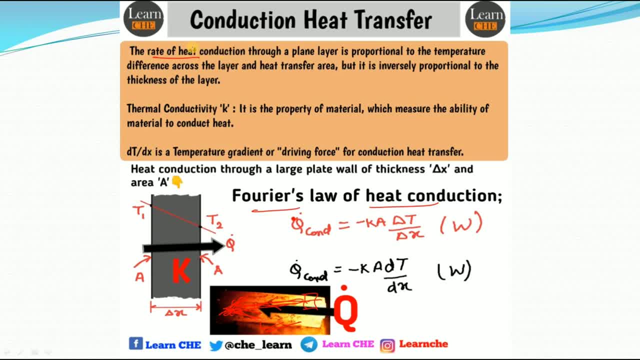 Fourier's law of conduction say that the rate of heat conduction, that is Q, through a plane wall is proportional, is proportional to the temperature difference. Temperature difference means delta T, which is a driving force across the layer and the heat transfer area. heat transfer area that is A, but inversely proportional to the thickness. Suppose thickness is here X. You can see here a plane wall where the direction of heat transfer is in this direction. 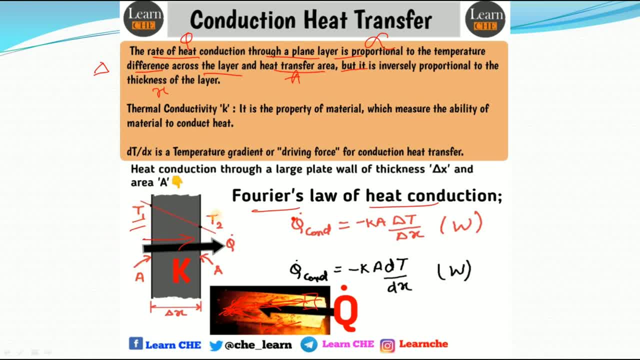 Okay, And here is a temperature is T1 of this surface and temperature T2 of this surface. heat is transferring in this direction because here temperature is T1 and here is temperature is T2 and if we suppose that T1 is greater than T2, then heat will transfer into this direction. Right, And this is the area, area of heat transfer. that is the area and this is a X, that is a thickness. Why I have written here delta X? because if I add a 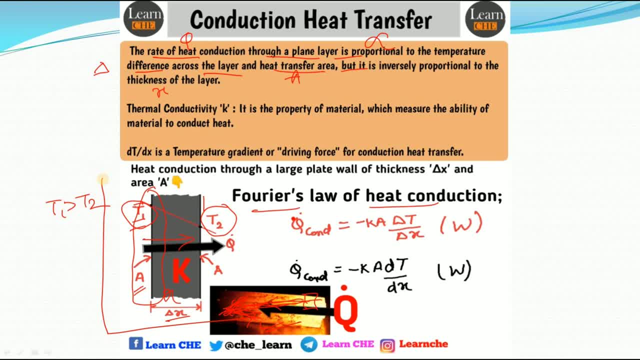 assume the length from the the axis, then it will be my, then it will be X1 and it will be X2.. That's why I have written here: delta X. Right, And this is a K. K is a thermal conductivity. I'll define it later here. What Fourier's law of heat conduction say, that the Q conduction means heat transfer rate of conduction is equal to minus K. A delta T by delta X. When I, when I want to replace this proportional sign, then 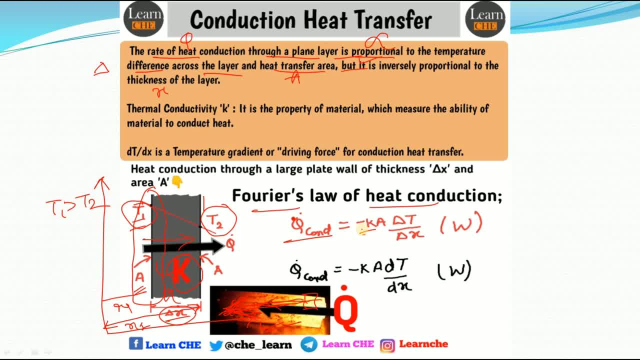 delta k, that is a, that is a thermal conductivity comes into the picture and it becomes k a, delta t by delta x. why here is minus sign? because heat is transferring from higher temperature to lower temperature. that's why here is minus sign, because when you will write delta t as a difference, then